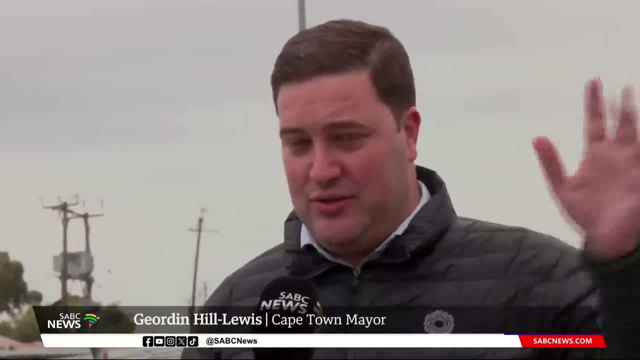 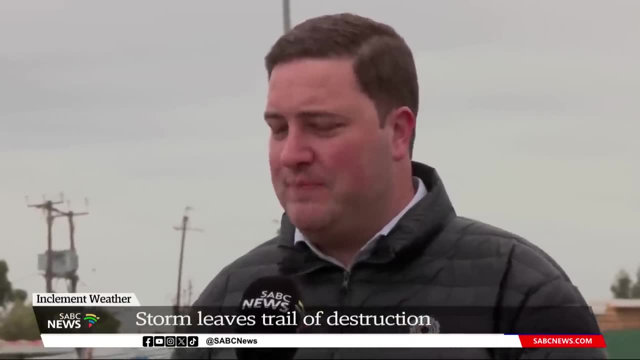 very strong and our city cannot use the crane trucks to get to the lines, the cables, overhead cables, unless the wind is is calm enough and safe enough for them to do so. So we really do ask people for patience, that the city teams will address those power outages as soon as they possibly can. 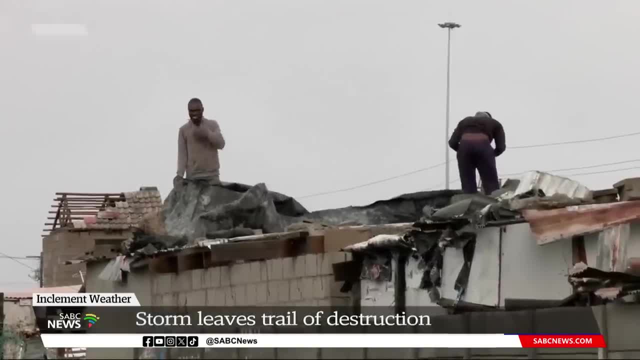 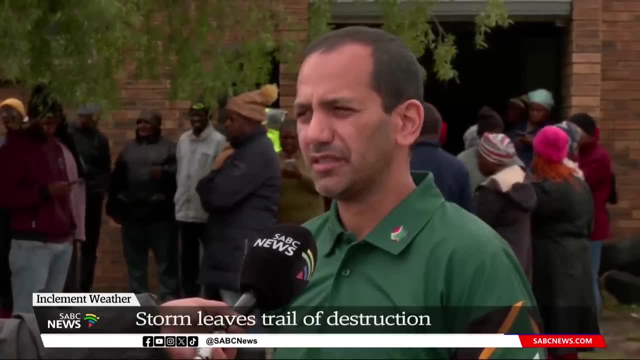 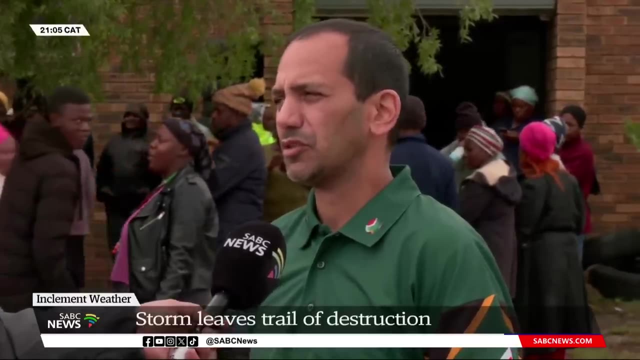 Aid organization. the gift of the givers says it's been inundated with calls for help from across the province. The main concern is the safety is number one, thereafter the humanitarian needs in terms of blankets Is blankets, hot meals, magic items, which we will be providing, and then, of course, once the weather subsides. 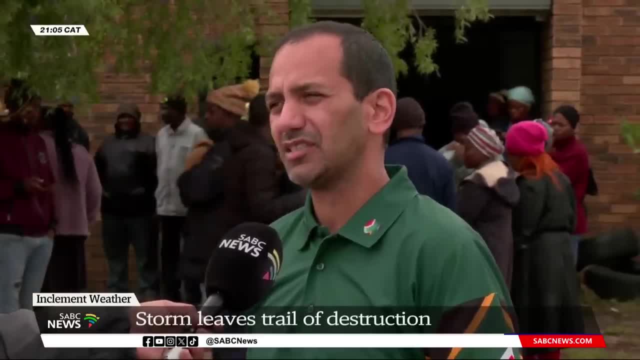 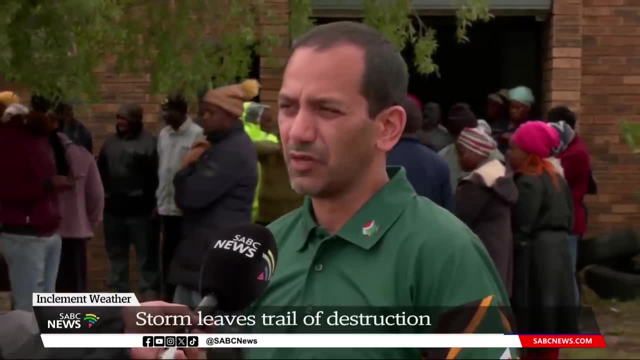 They would need some building material to rebuild the homes, But we could see the extra extents of damages as which and with, as you correctly said, the range is not coming down 100% yet, But it is rain predicted for later on, in terms of 100 miles of rain predicted. 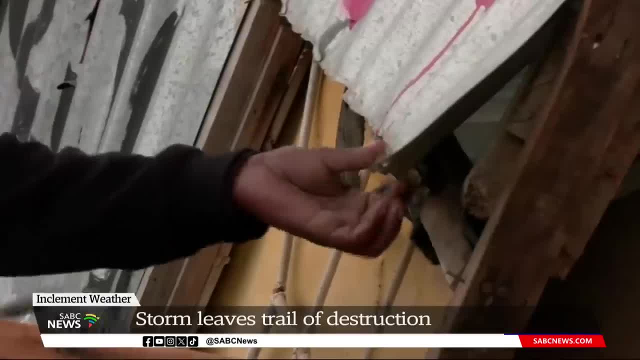 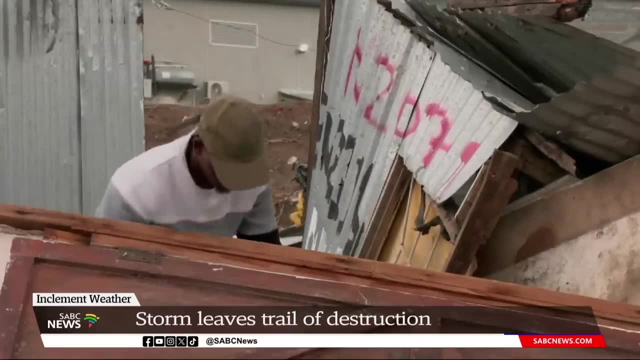 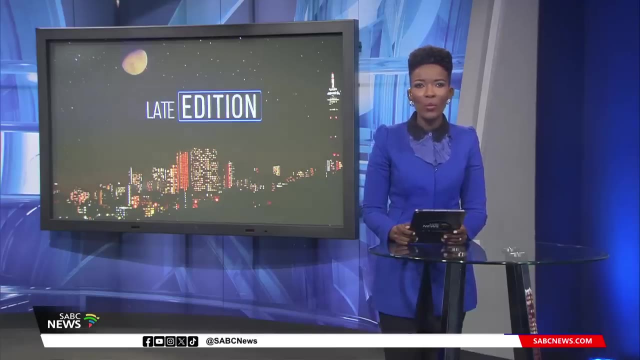 So it will. it will be intensifying. Oh, it's 24 hours. Assessments of storm damage and mopping up operations are ongoing. Vanessa Pooner, SABC news, Cape Town. Right, Let's bring in some reaction on the from the city of Cape Town's impact of the adverse weather conditions. 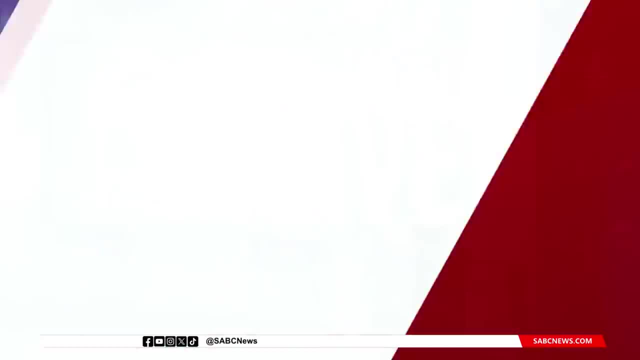 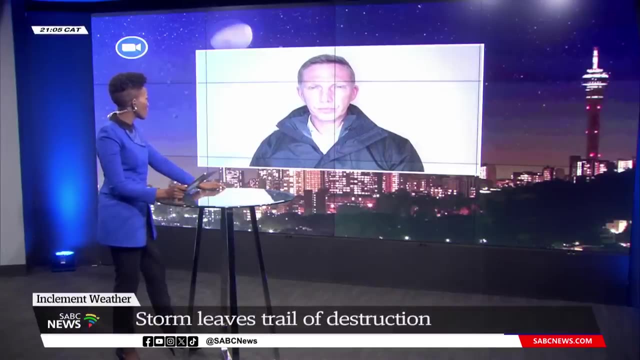 We're joined by the city of Cape Town's MMC for safety and security, JP Smith. a very good evening to you. Thank you so much for your time, JP. the inclement weather has wreaked havoc across the city. Let's perhaps start off with an update on the latest developments on the ground this evening, as you and I speak. 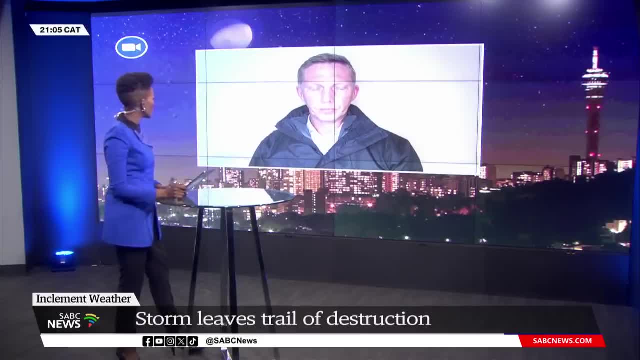 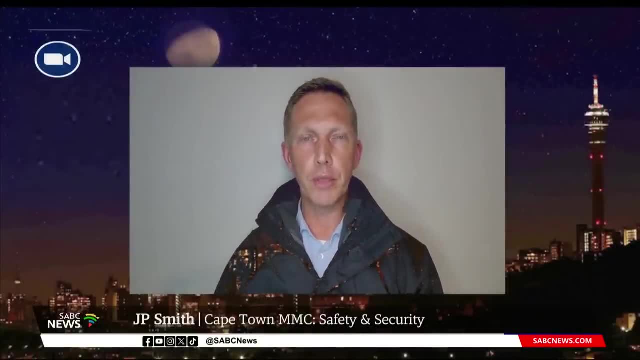 More so after learning of a loss of life. We're joined by the city of Cape Town's MMC for safety and security. JP Smith, a very good evening to you, Absolutely. our disaster management teams have been working with all the different departments over this day. During today, we had very few additional incidents. Mainly we were dealing with mopping up from the damages of yesterday. 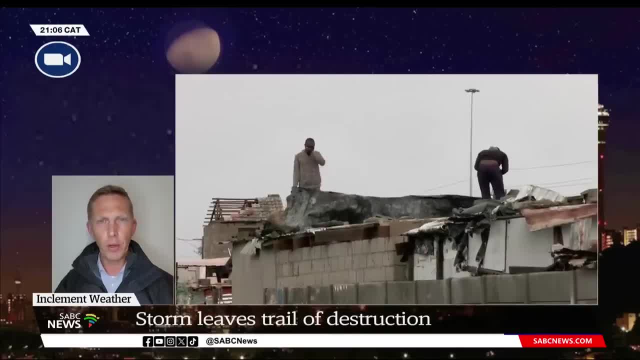 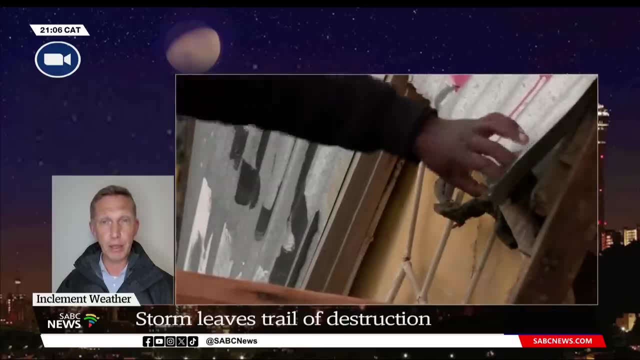 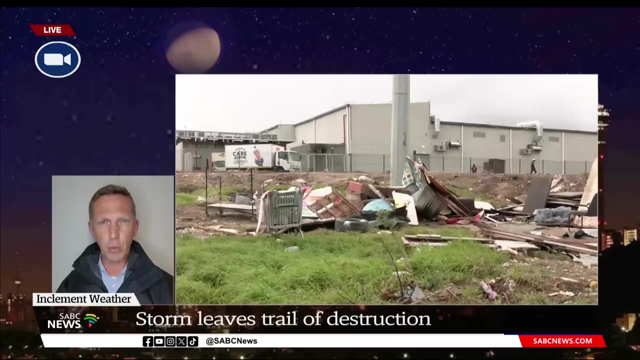 Afternoon and last night we had extremely heavy rainfall, well beyond the normal winter rainfall levels. We had a storm like this in September last year as well, So these extreme weather conditions truly put our services to the test, and we had howling winds of 60 to 80 kilometers an hour. 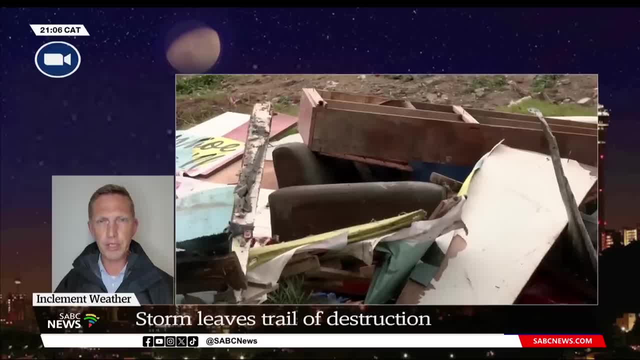 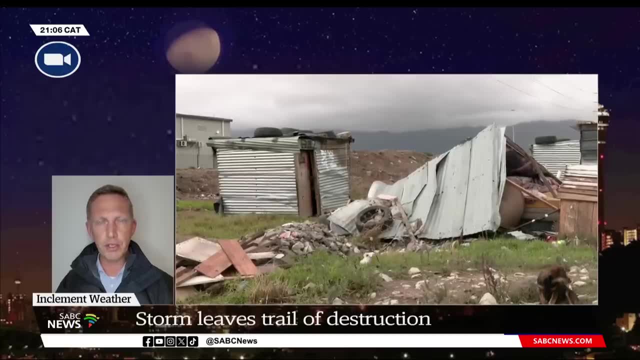 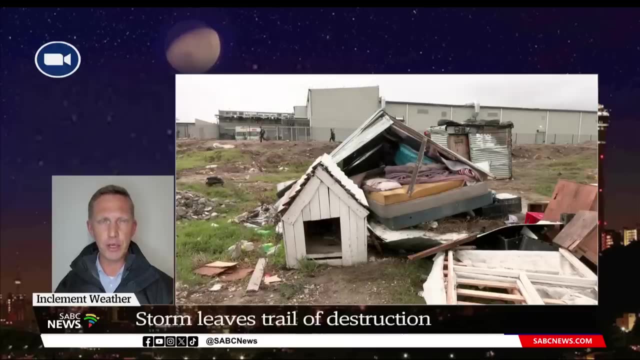 At some places due to the localize topography that was even more severe, that lead To the kind of damage you see in these clips with structures. Myself in the mail were one site during the day, visiting different areas To see what our disaster teams are doing. our informal settlements management officials were engaging with people to see where start to kids were possible. 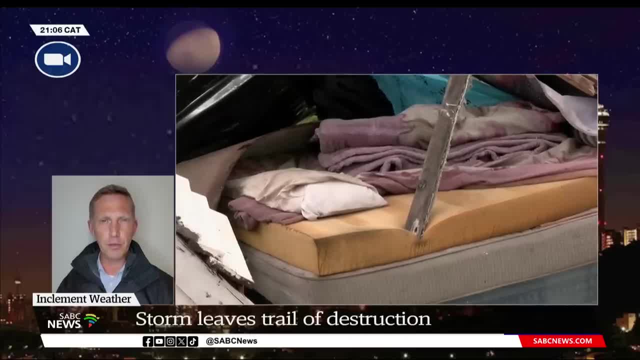 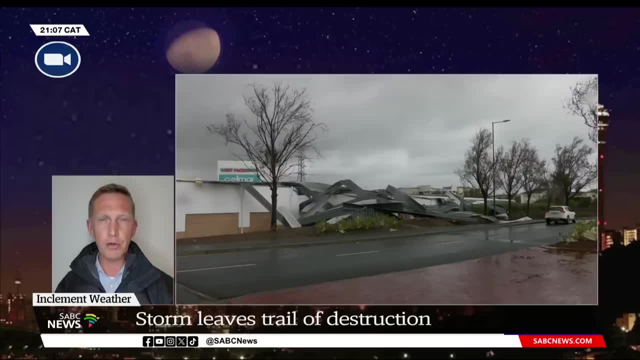 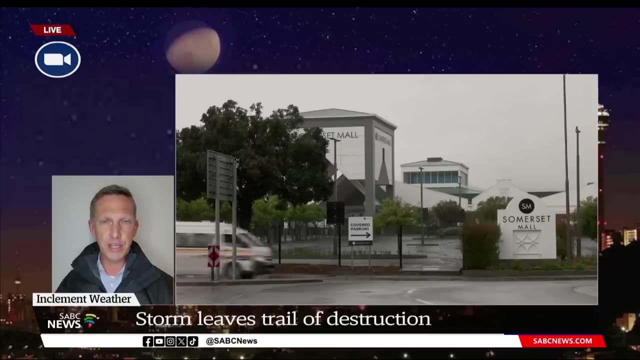 possible. Various relief agencies, including Give to the Givers and Mujtadafin and others were assisting with relief. We had done a call for donations already on Sunday, with various companies and corporates coming forward with donations and Checkers 6060 making a. 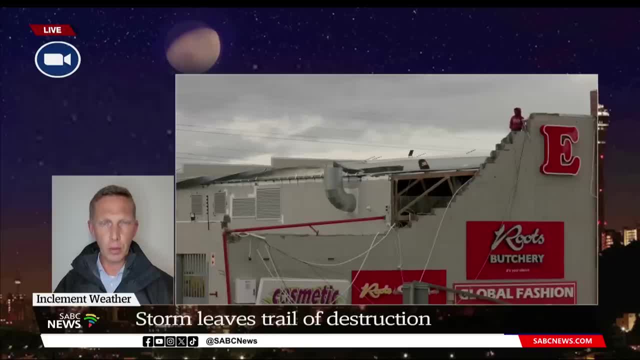 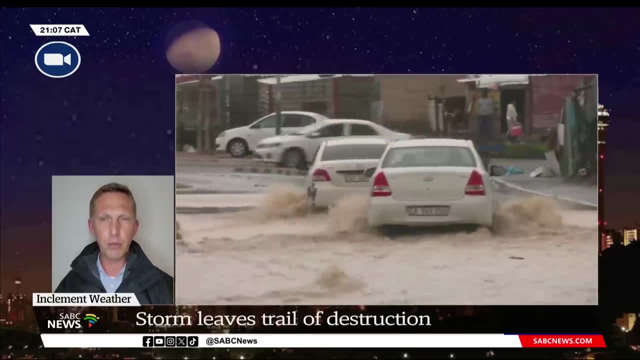 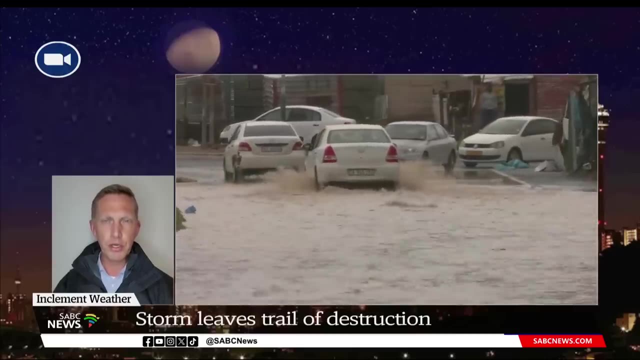 donation option available on the app. So we were able to start doing some relief materials today, and thanks also to Peninsula Beverages and the Grand West Hotel and Grand West Casino and others who contributed. and then our teams were busy, as the Mayor also alluded with. 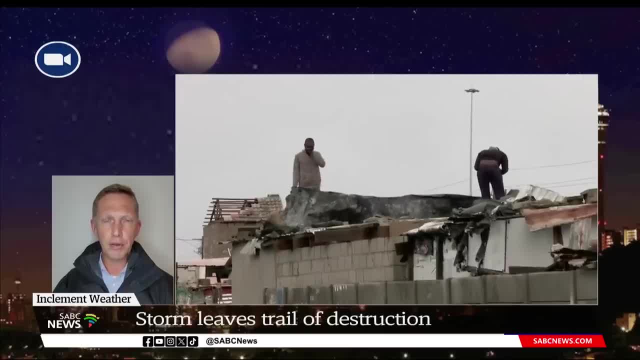 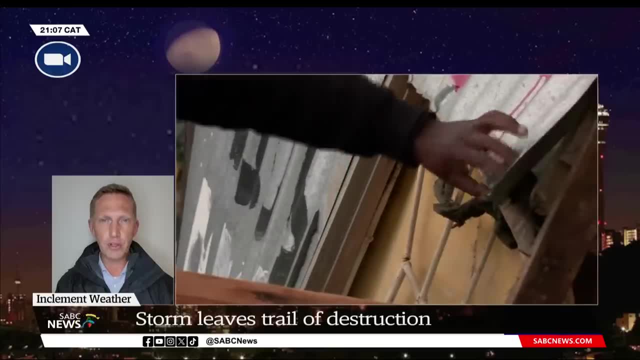 the electricity outages. by this afternoon, Early this afternoon, 10 of those 30 outages had been corrected. There are working currently on 20 that are still open and that they are attending to. Many of those will be fixed during the night, especially if the wind gives. 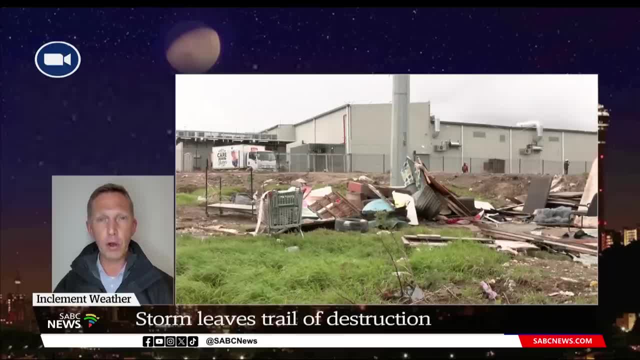 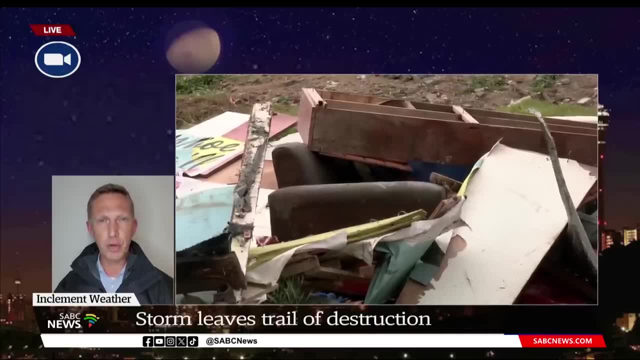 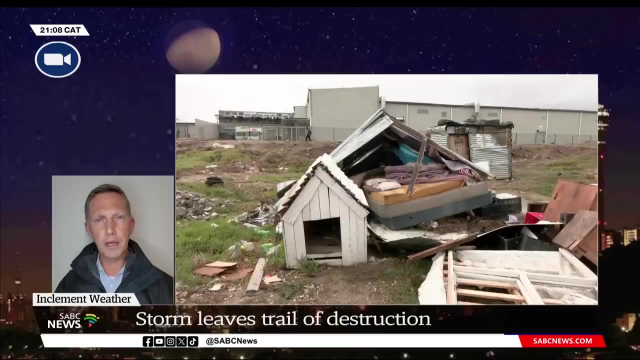 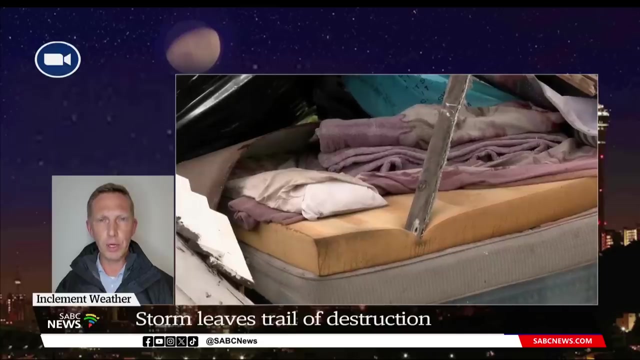 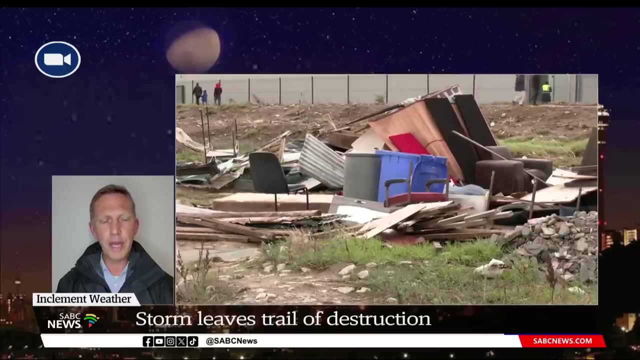 us a bit of a break and the pumping out of localised flooding blasts and thunderstorms happen. And then, of course, the other piece of the issue is the industry. So right now we have emergency risk assessment and we have managed to manage that through ourιοvership initiatives, and we all know that we are in a very difficult situation. We are tired and exhausted. I think it's really important to make sure we are in a safe state and we have all the resources we can to do that. I'm going to turn it over to the Board of desarmeh. 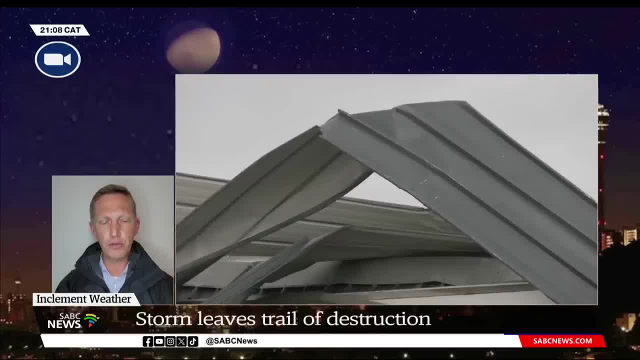 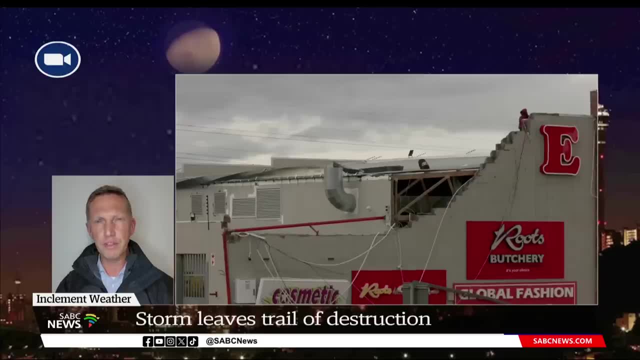 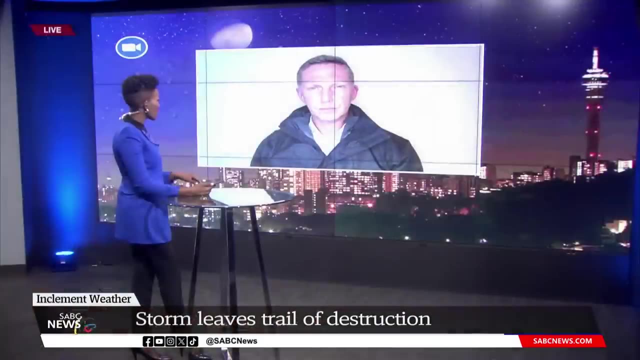 Thank you very much on the on the roads, with fallen trees and otherwise, and i think that is uh has also stretched into capacity. so in total about 2779 structures that were affected where we were giving assistance today with that extent of infrastructural damage, we also understand that uh some 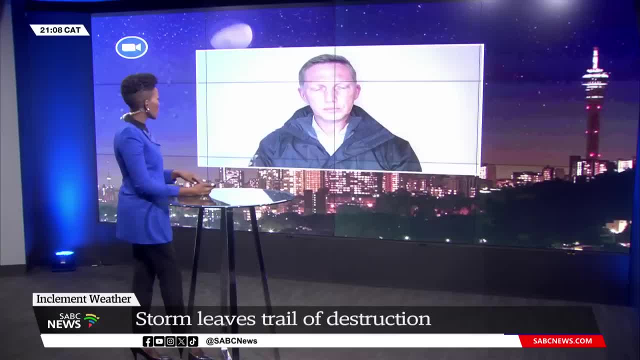 structures in in nomzamo have been affected and people, of course, being displaced. where are they being housed this evening? and and also perhaps talk a little bit about the areas which have been hardest hit, as you try and bring some sort of normalcy. generally, those were in the far southeast. 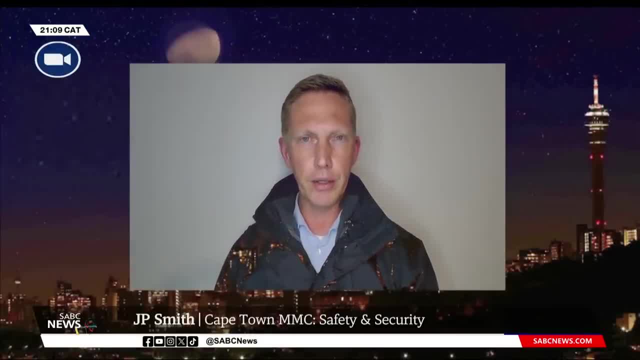 of the city, those closest to the overburg and cape wineland. that's where the wind was most severe. most of this damage is wind damage. the electrical outages were caused by trees falling on lines and parts of structures or other debris becoming wind blown, especially sheeting of. 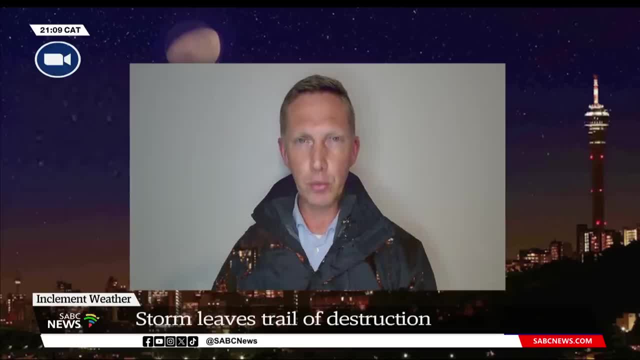 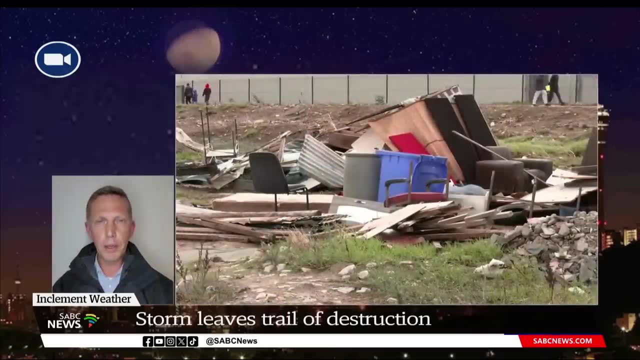 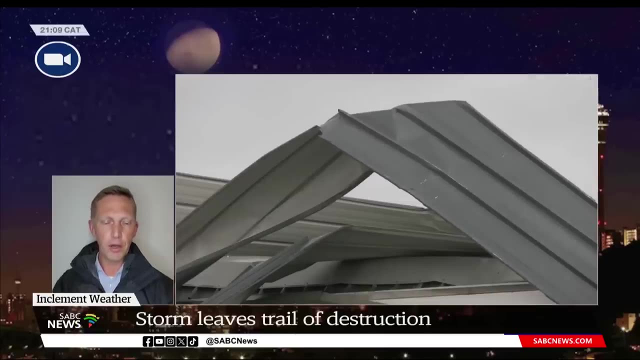 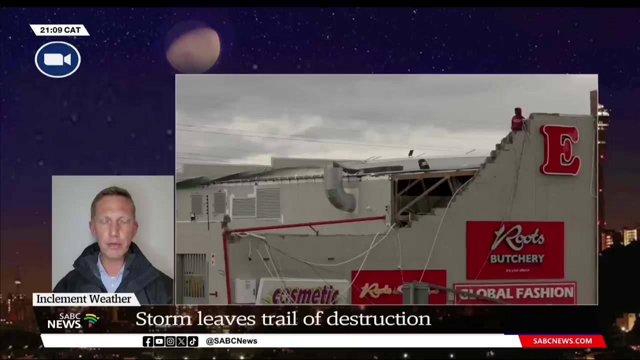 informal structures that became airborne and tangled with wires or cut electrical cables. so that's given the electricity department most of their work and, in terms of the areas affected, namzama probably has the largest number of structures: sunda village in bolila a and toronto- from a single structure slightly damaged to a small network of structures. 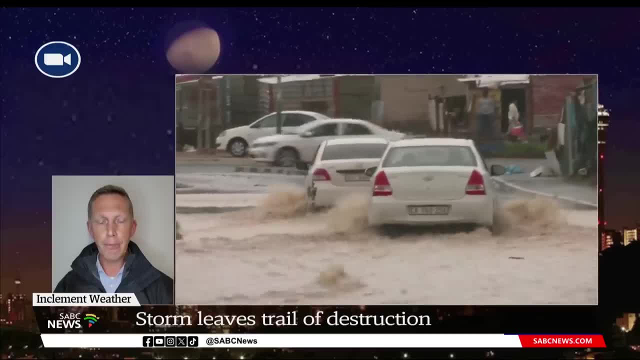 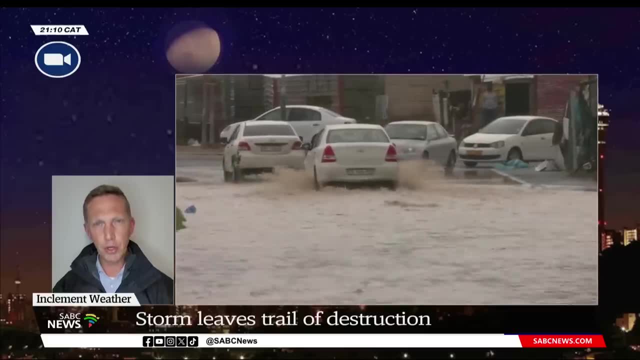 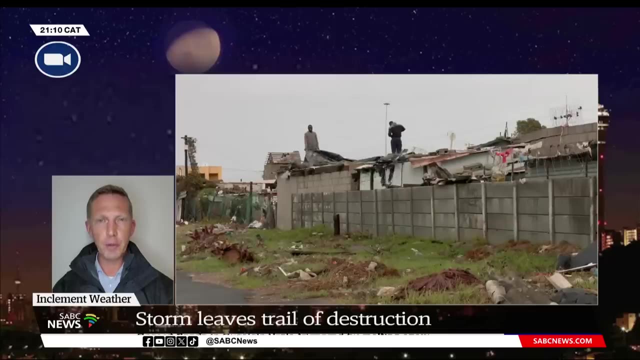 a large number of these was left to reserve in the form of a normal settlement at quite a number, and these range from a single structure slightly damaged to quite a large number of structures- up to 720 in the one area and, as i said, around seven 2779 structures, ranging from a very slight 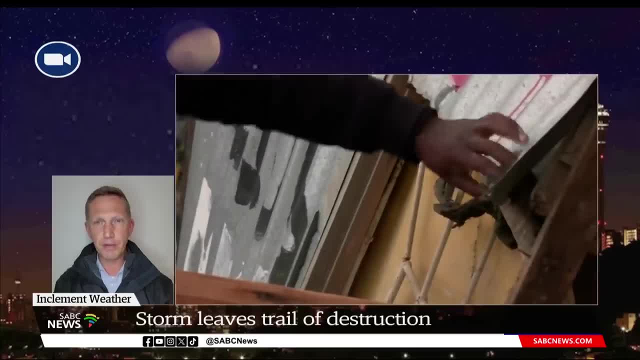 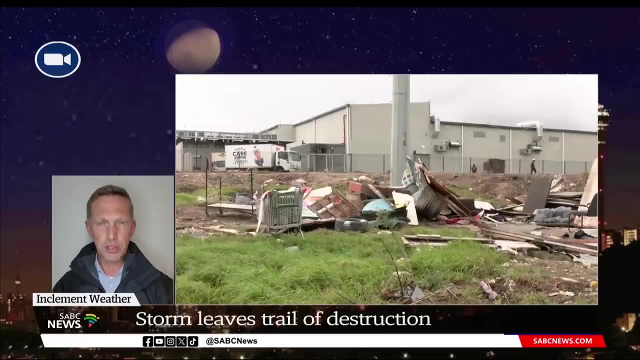 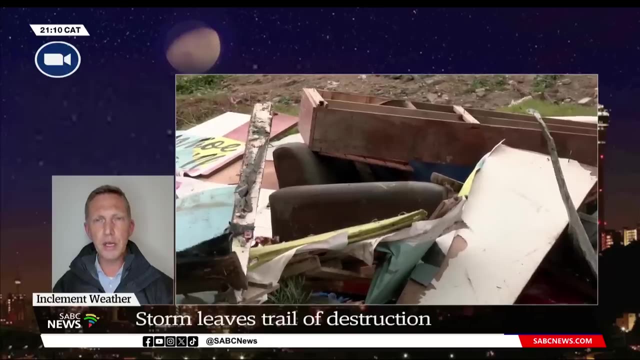 damage to to completely torn down by the wind. uh, with relief options, we generally are trying to called on an activated community organizations, churches, other faith-based organizations- to assist people with some shelter overnight. The challenge being with opening community halls is that very often the next day when those community halls and people need to leave, 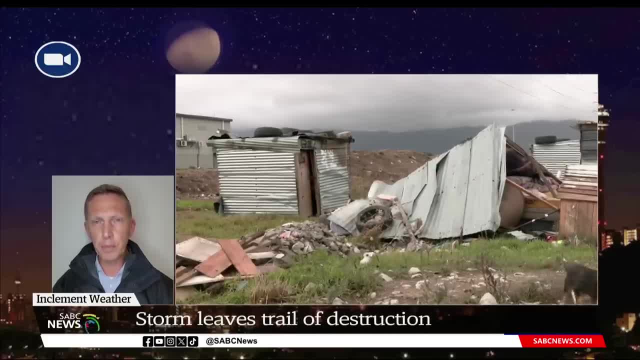 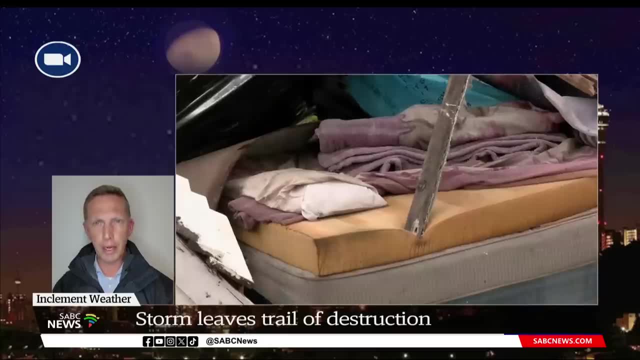 they will decline to do so And that community hall is then lost in perpetuity to community access, which creates a great deal of anger, And this unfortunately relates to how the courts interpret the PIE Act, which creates additional challenges for us there. But where we were? this? 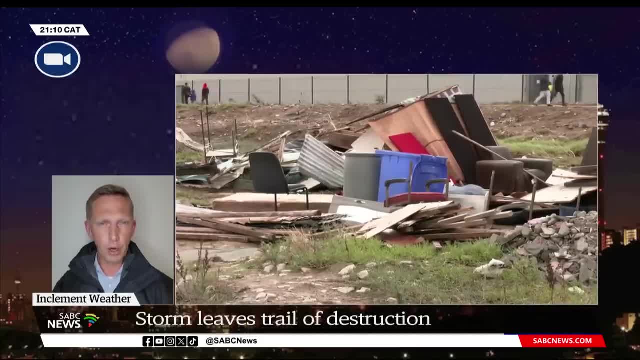 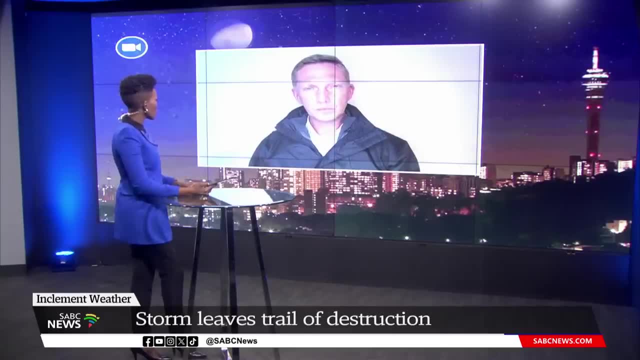 afternoon, people were either rebuilding or had, by and large, found accommodation with others. We also understand that some schools, as a result of this weather, had to be closed. Is that something that will continue up until tomorrow? What are the conversations around schools? 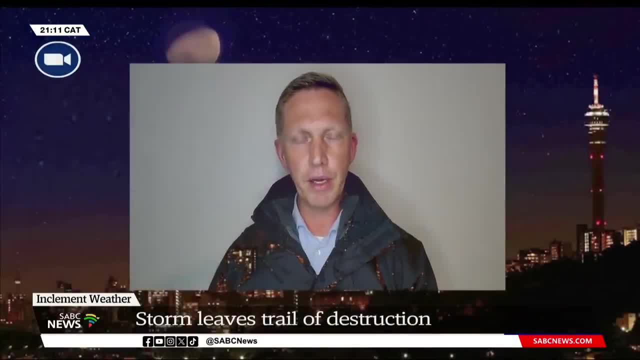 So the Premier, Alan Windy, has been having discussions and has asked for briefings for our staff. We participated in one early this morning and during that various assessments were done between the city and the province and other municipalities surrounding us. activation of mutual aid agreements between us And, in that regard, the 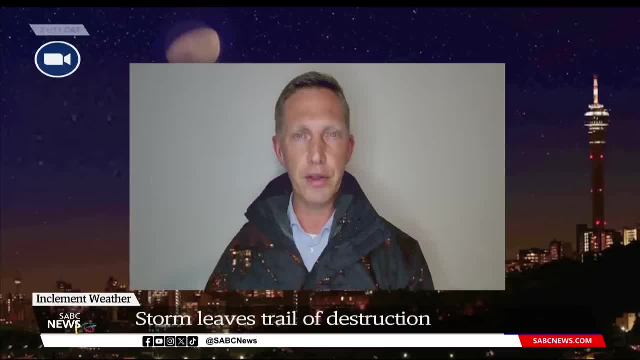 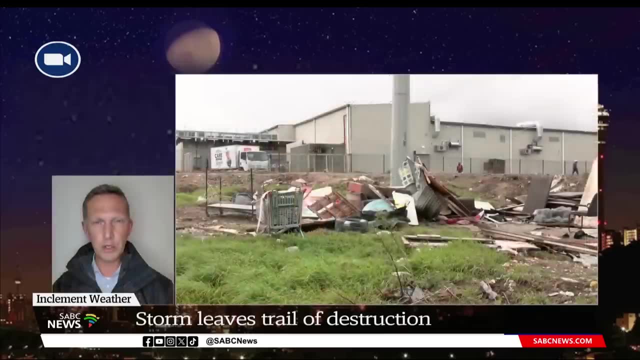 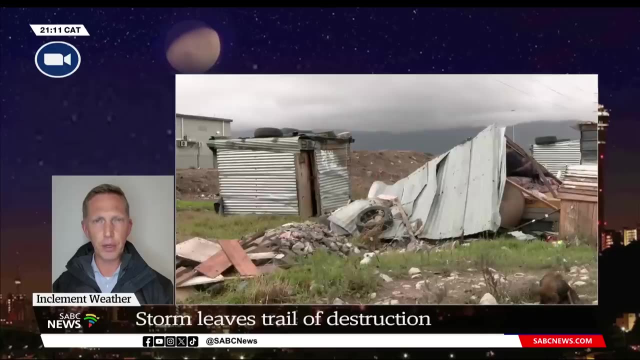 Premier then closed the schools on the eastern side of the city and the Alderberg side, Somerset West and surrounds, where the weather was extremely severe and wind speeds became very intense, And schools within the Cape Winelands and Overberg. 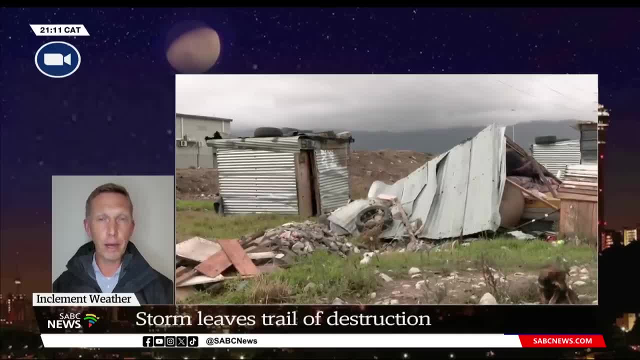 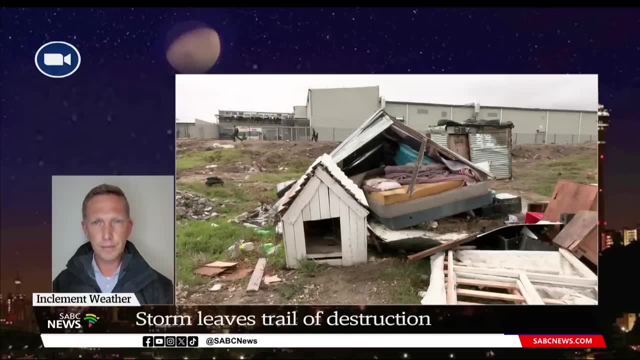 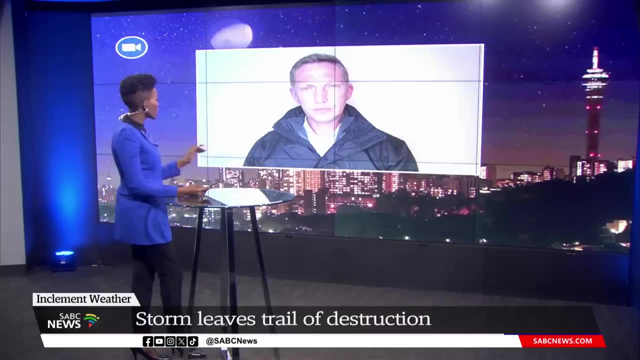 the rest of the city was not affected in that regard, Although I think learners had in some cases, had a challenging time of getting to and from school. today, And you touched briefly on you, know what happens when people are housed in churches and all of 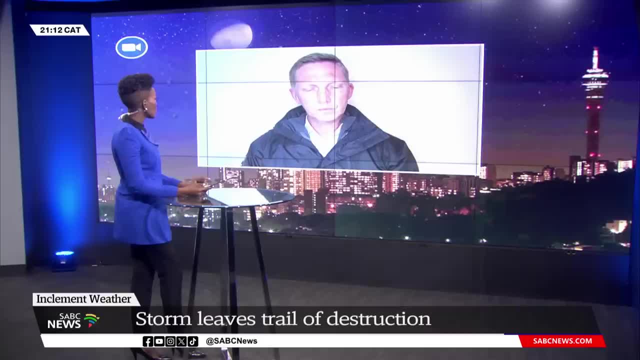 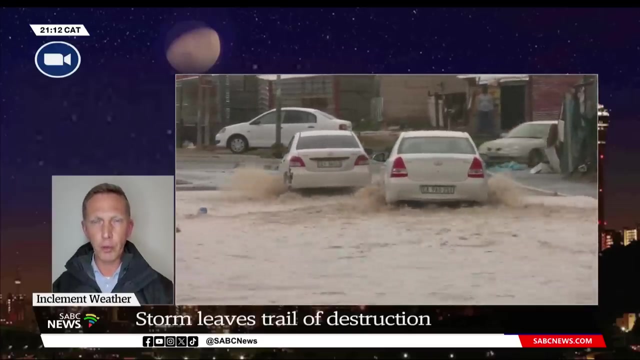 those serious challenges? What assistance will be given to those who may have lost identity documents and serious paperwork? Are you working with other departments to assist them at this stage, Or is it still too soon, as the inclement weather continues So before the extreme weather occurred over the weekend even as far back as last week, on Thursday? 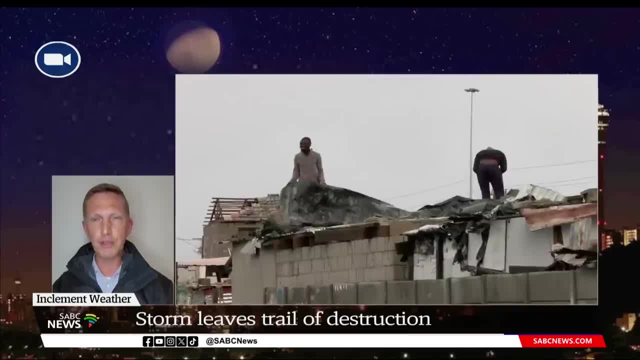 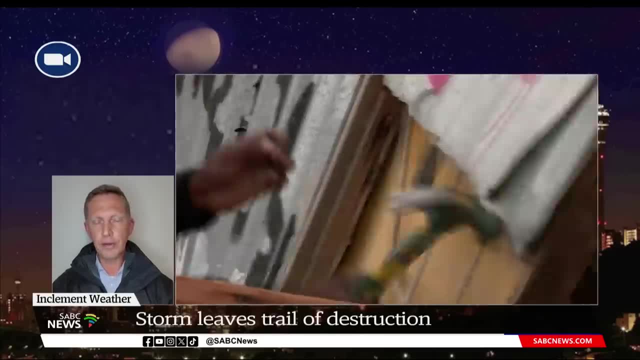 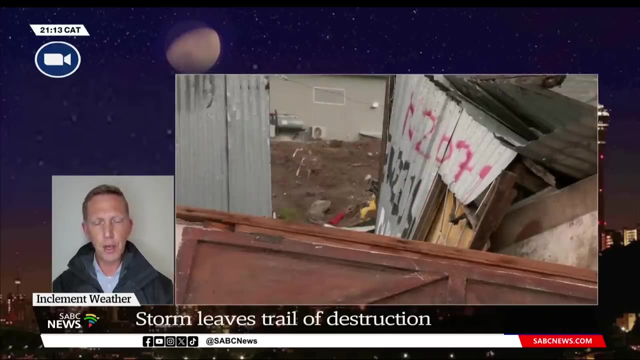 we started meeting with all the different agencies and putting our preventative measures in place, But we pre-activated some units, like the dive units and the rapid water rescue units that were in our fire and emergency rescue services. We then started convening over the weekend already. 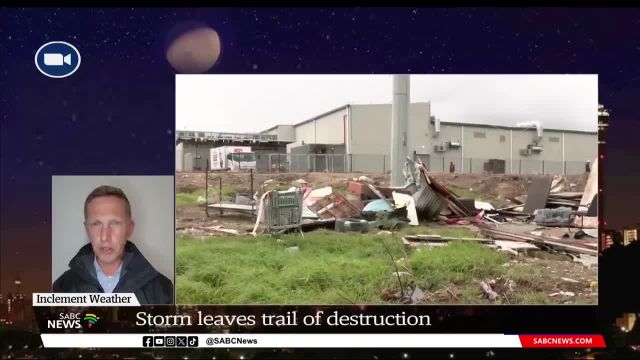 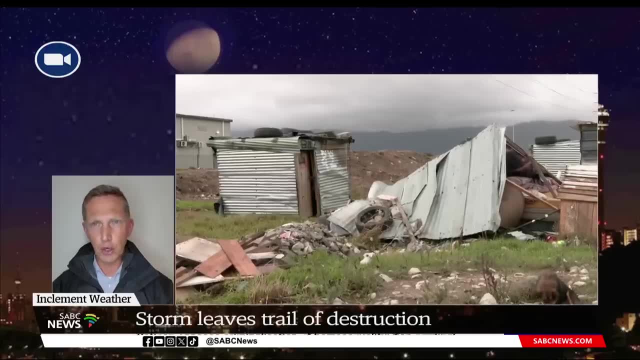 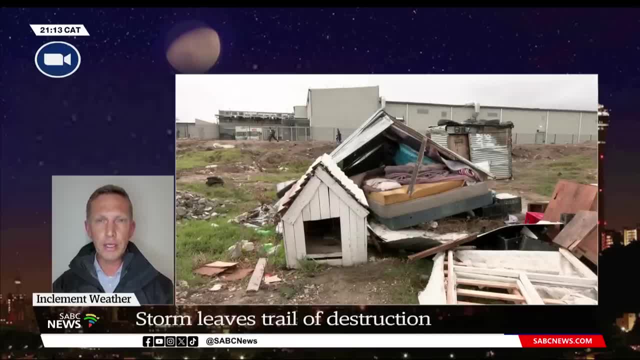 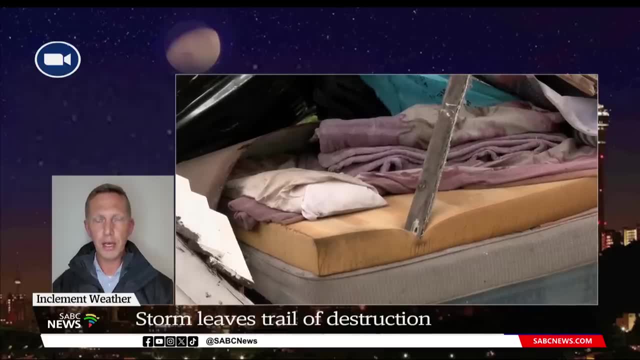 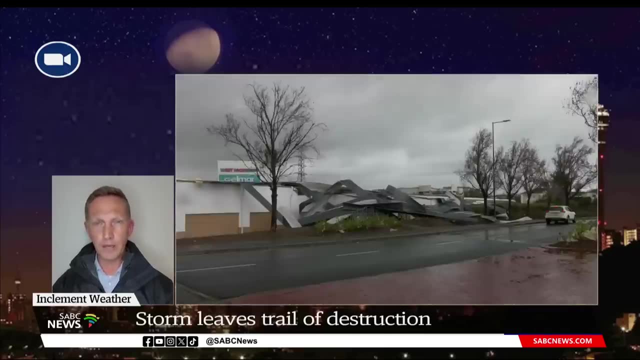 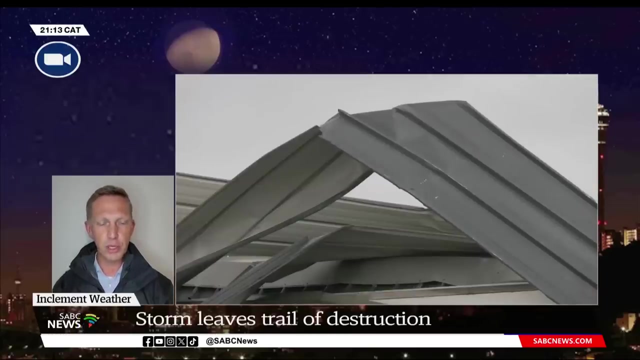 And various disaster coordinating information in infographics and otherwise, through social media, through your neighborhood watches and otherwise, so that people could prepare and be ready and new to contact for what. And then over the weekend we activated the disaster operations center with all the different departments, including SASA, DSD, urban waste management, water, electricity.